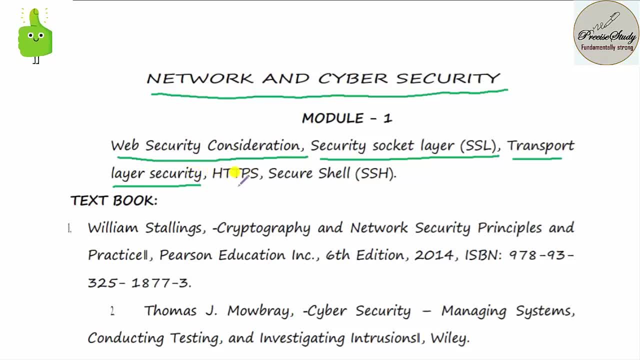 In initial days the website will be having HTTP, but nowadays the website will be having HTTPS, nothing, but it is a secured one, and we will be talking about secure shell, that is, SSH, The topics that is SSL and transport layer security. secure shell is very, very important. 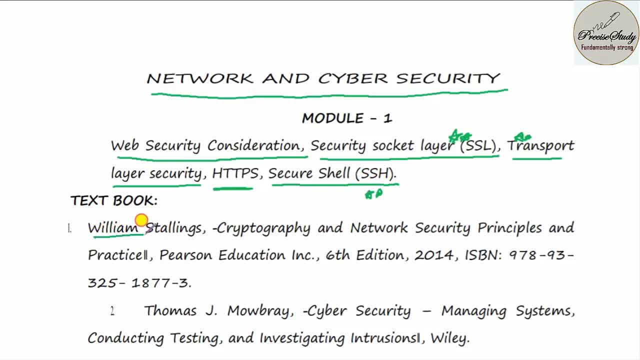 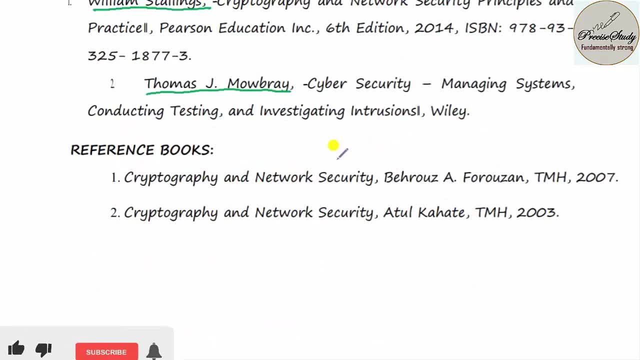 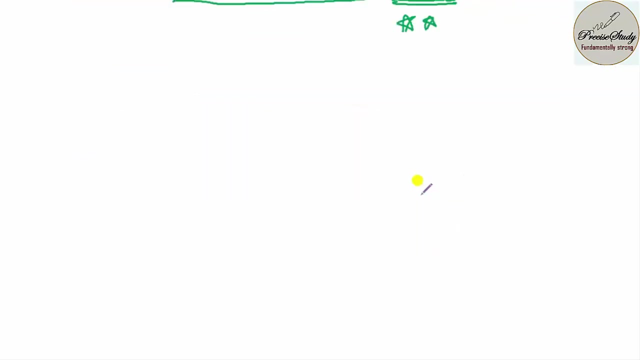 You can refer to the standard textbooks. The first one is William Stallings and the second one is Thomas J Morbain. Also, for further information, you can refer to cryptography and network security by Ferozel, and the second one is cryptography and network security by Atul Kahate. This, Atul Kahate, is a layman language author, So once, if you are reading, you will be in a position to understand each and everything. 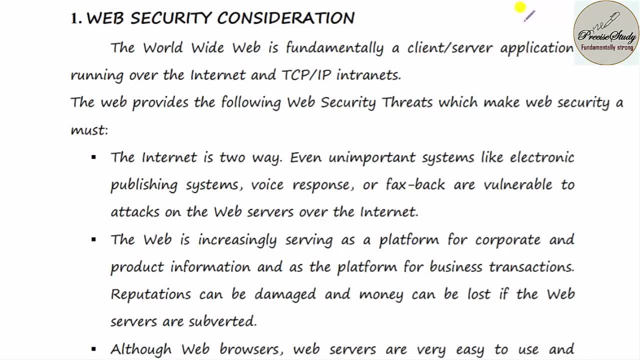 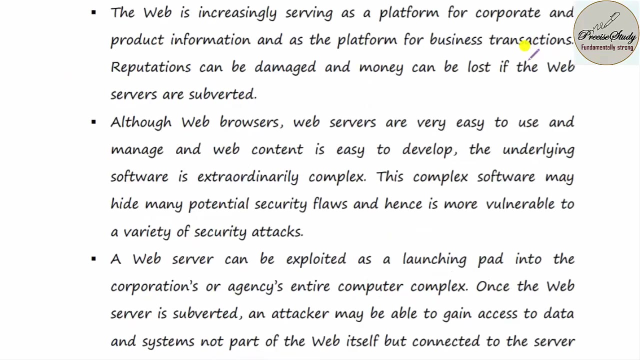 Now, what do you mean by web security consideration? In olden days, all the important data or documents we used to keep in a locker, but nowadays what you are going to do is we are going to completely depend on cloud. Say suppose, if your data is getting hacked, then it is a very much critical task for you in order to retrieve the data. So what you are going to do is you are going to store the data in a trusted website. Example is Dropbox, Google Drive. 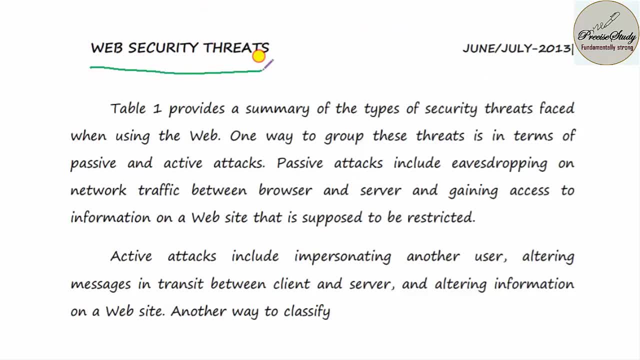 We have two variants of web security threats. The first one is passive attack and the second one is active attack. Say suppose, if so, X and Y are communicating via communicating channel. So what Z will do? Z will be very much eager to know what X and Y are communicating. So if Z is reading the data, if he is only reading the data, then he is doing passive attack. 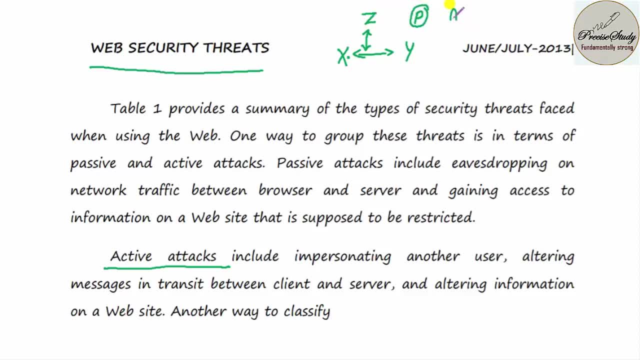 If he is reading the data and if he is modifying the data, then it is an active attack. Say suppose, if X wants to convey some information, he will be putting his information on the channel. So, before reaching Y, what Z will do is Z will read the data and without modifying the data, 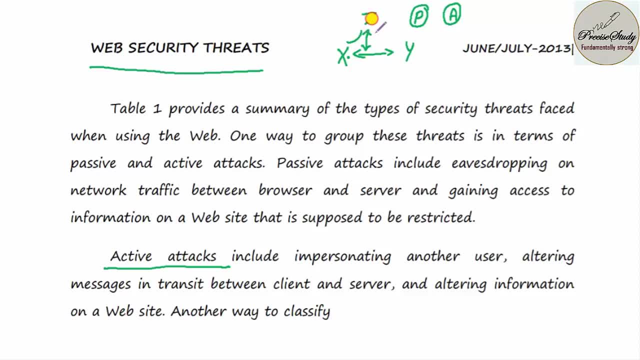 if he is sending the data to Y, then it is a passive attack. If he is reading the data and if he is modifying the data, then it is an active attack. Upon modification, what Y will be thinking is the message as sent by X. he will not be coming to know that the message has been modified by Z. 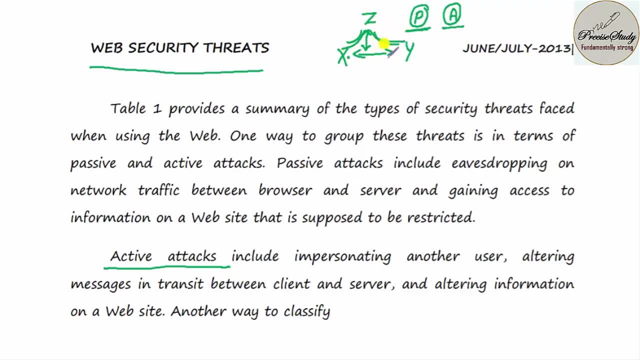 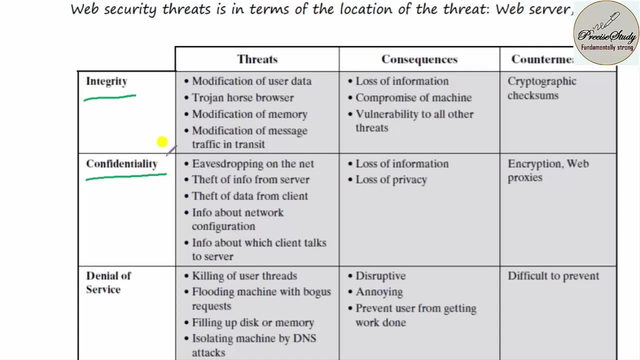 So this is a severe threat in the case of communication. So these things are very, very important. They may ask you write a short notes on it. They may ask you write a short note on integrity, confidentiality. what do you mean by Daniel of service? what do you mean by authentication? 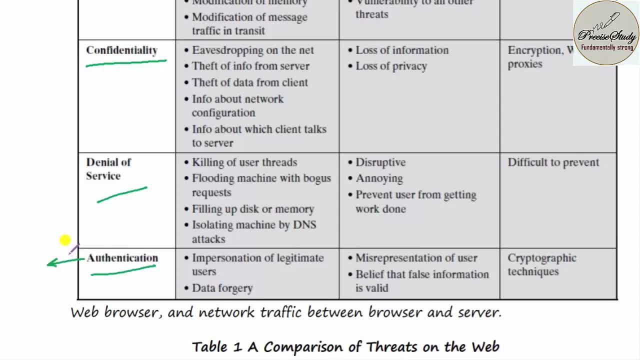 Now, if I am talking about authentication, say, suppose you want to log into your gmailcom, or if you want to do any transaction in a bank or internet banking. if you want to do, At that time they will be asking for two-step verification. nothing, but they will be sending an OTP as well, as you should know the password also. 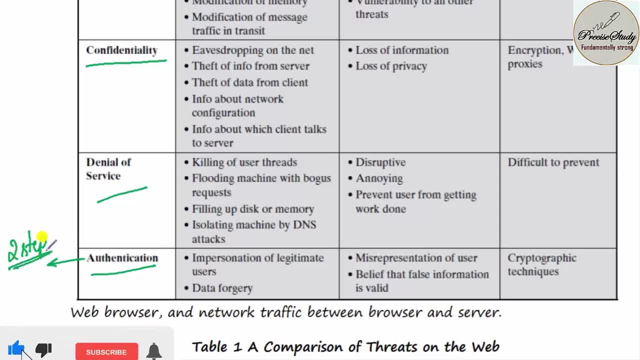 So password is the first step, verification. Second step: verification. So they are gaining somewhat security for your account. What do you mean by Daniel of service? Say suppose you have installed some particular application on your mobile. You are having 1 GB of memory but the application was taking, say suppose, some 10 MB of memory. 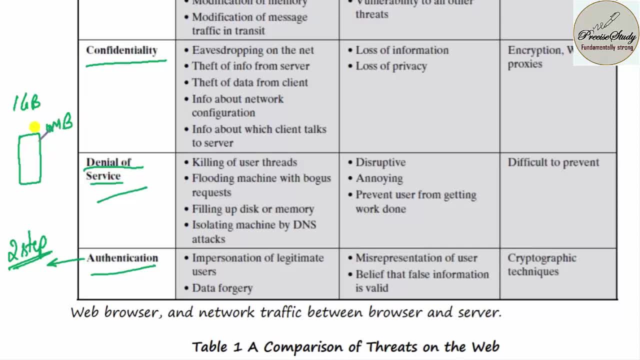 As days proceed. what this application will be doing is it will be overloading your mobile At that time. This application is a culprit, So it is something like it falls under filling up of disk or memory, So it is a consequence. 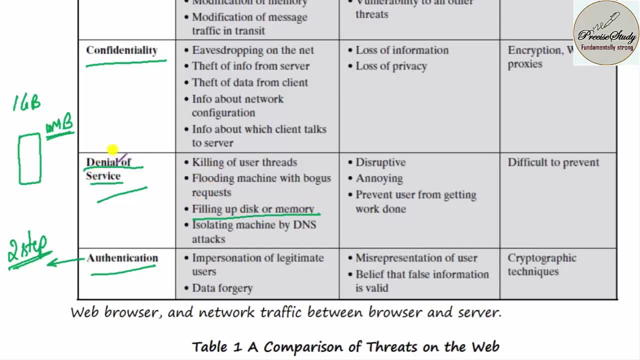 So what you have to do is every time you have to check for the cache memory. Also, you have to check for how long your application is running at the background and how much internet it is consuming. So this is one of the security measures what an Android user or an Apple user can adopt. 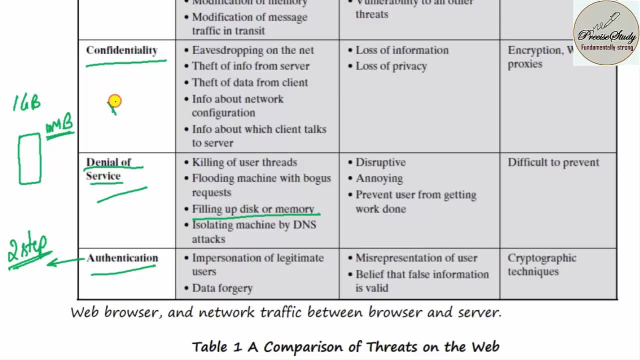 What do you mean by confidentiality? Say, suppose if X is sending the data to Y over a network, So this network will be controlled by some persons, So they have to give a confidentiality, nothing, but they should be 100% sure that none of the hacker will be accessing their data. 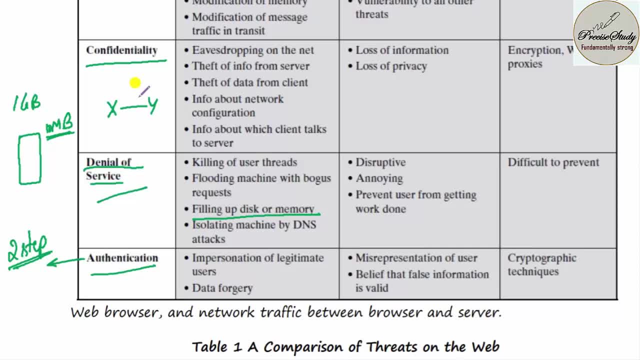 So that much of secureness if they are giving, that determines the confidentiality. If you are not having any confidentiality, then there will be a loss of information, Also loss of privacy And loss of trust. And what do you mean by integrity? 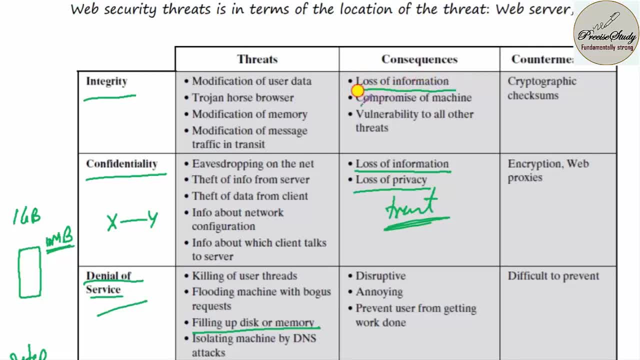 The consequences of integrity are loss of information, compromises of mission, vulnerability to all other threats. So what are the threats with respect to integrity means Modification of user data If I'm telling that tomorrow is holiday, if the message is circulated as tomorrow is working day and you have to work. 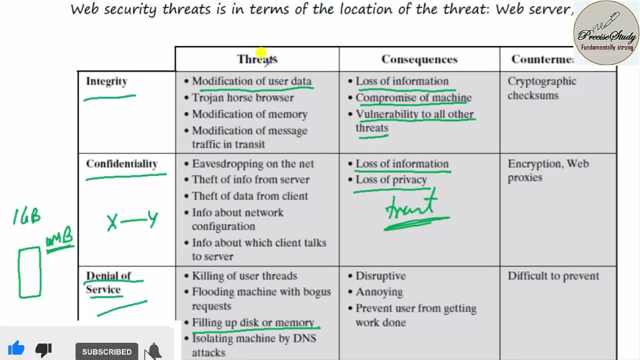 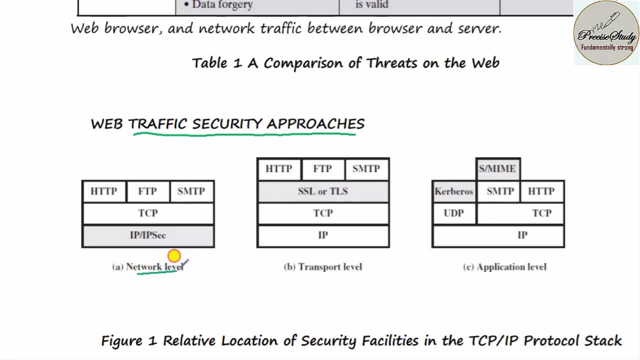 for one hour extra, then this creates lots of discriminating among employees. trojan horse, browser modification of memory, modification of message, traffic in transit. So all these things you should know. The web traffic security approaches are network level, transport level and application level. 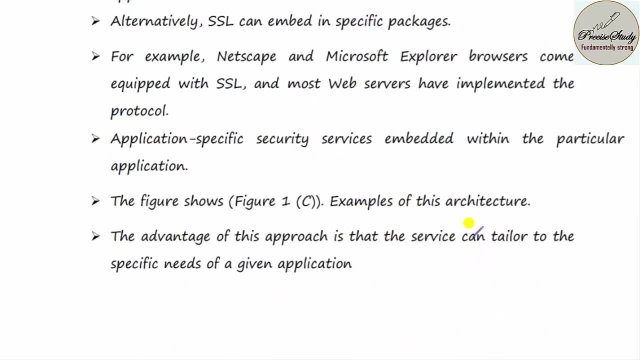 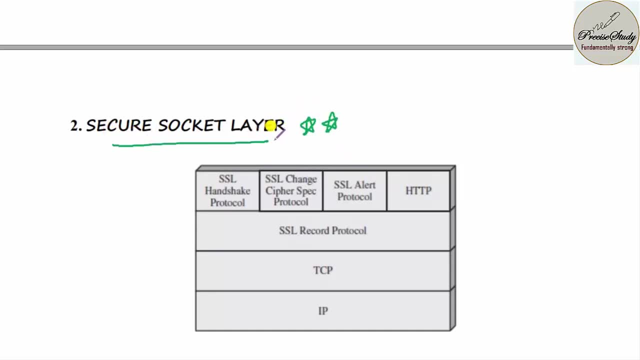 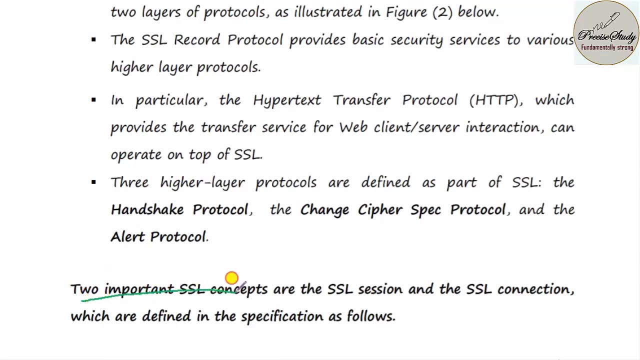 All these things you have studied in TCP IP protocol. Next, let us talk about secure socket layer. This is very, very important. They may ask you to write a short notes on secure socket layer And they will be also asking you what are the two important secure socket layer? 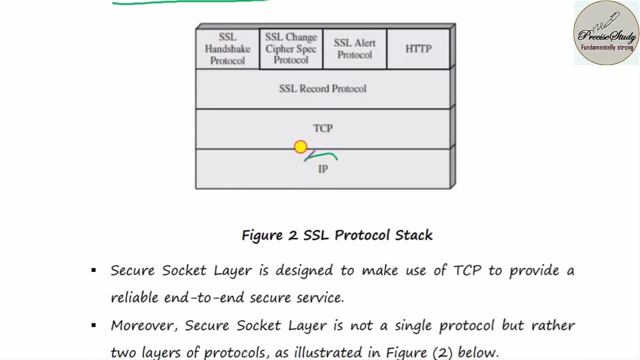 Now, what do you mean by secure socket layer? In the first layer you will be having Internet protocol, And the second layer is TCP protocol, And the third one is SSL record protocol And the fourth one? they have bifurcated into four groups. 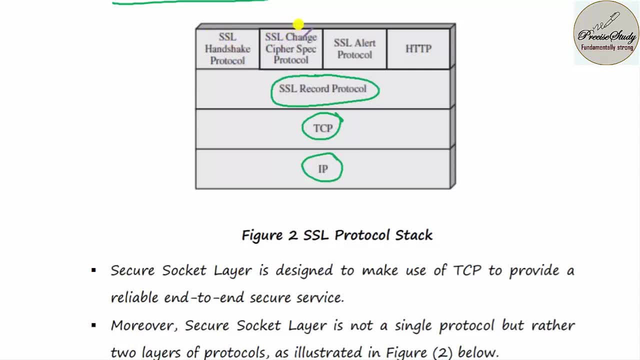 The first one is SSL and check protocol. The second one is SSL change cipher specification protocol. The third one is SSL alert protocol. The fourth one is hypertext transfer protocol. What do you mean by secure socket layer? It is designed to make use of TCP to provide a reliable end-to-end secure service. 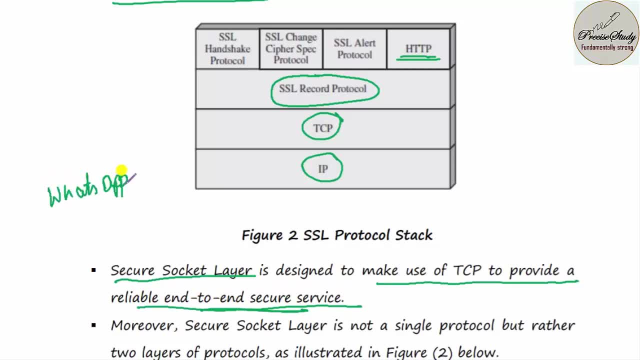 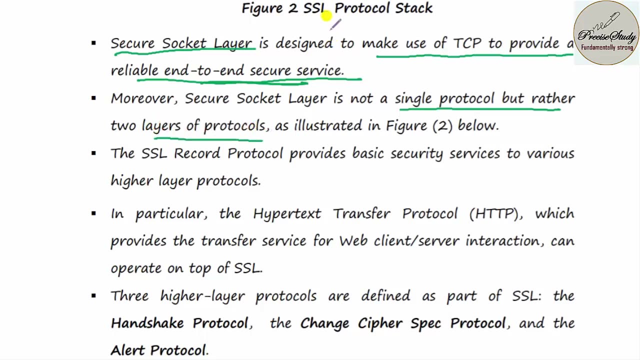 Example is WhatsApp, So first time if you are messaging, you'll be getting a message stating that end-to-end secure communication has been activated. Moreover, secure communication is not a single protocol, but rather two layers of protocol, as illustrated in the figure two. The SSL record protocol provides basic security. 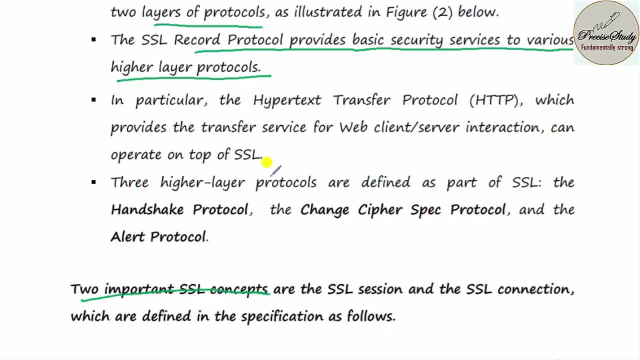 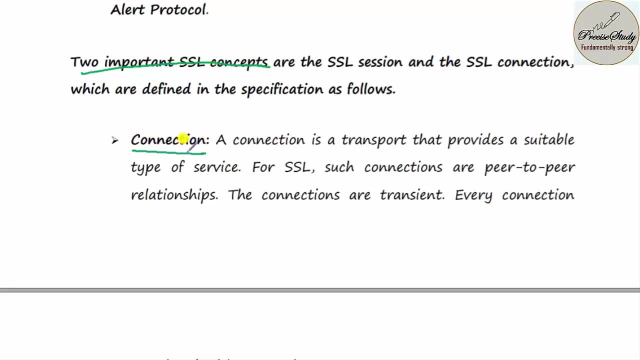 services to various higher level protocols. The main thing is loss of data. should not be So. what are the two SSL concepts is the first one is connection. What do you mean by connection? Connection is a transport that provides a suitable type of information for SSL. 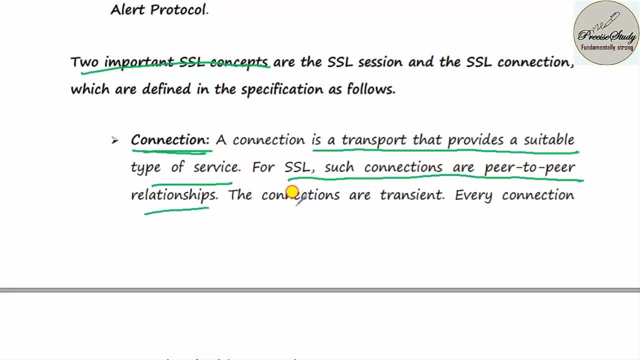 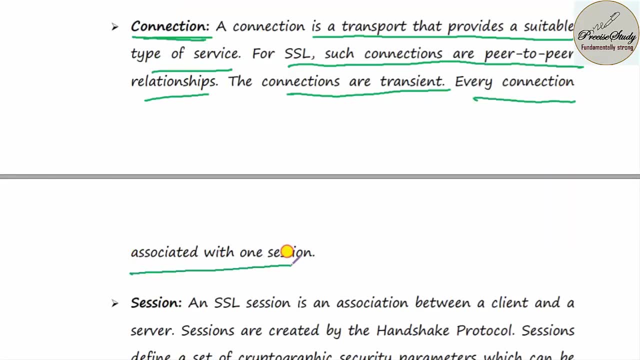 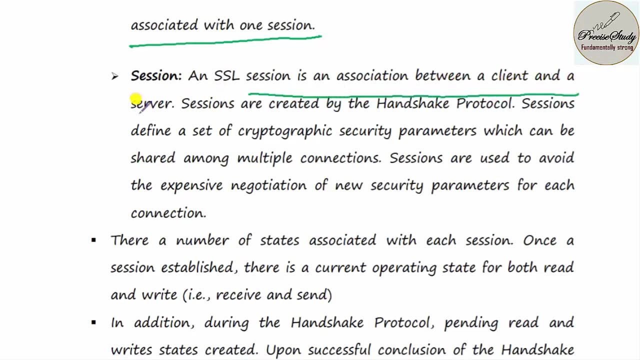 Such connections are peer to peer relations. The connections are transient in nature, So every connection will be associated with at least one session. So what do you mean by a session? An SSL session is an association between a client and a server. 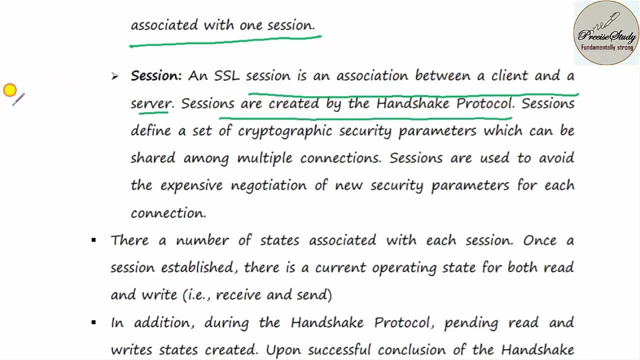 Sessions are created by handshake protocol. Say suppose, if you want to interact with one more person via phone call, So you'll be making a telephone ring for the second person. If the second person is busy, he will not be responding to your call. 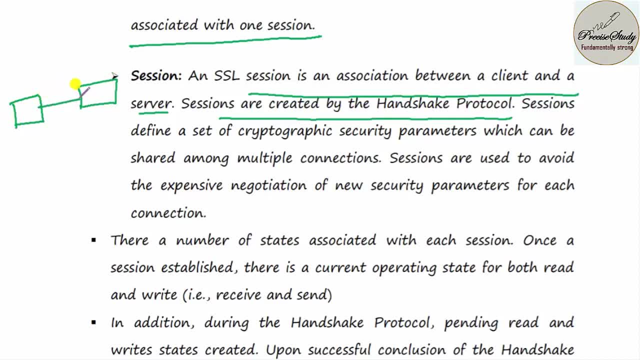 So first, what the operator will be doing is say, suppose, if user is busy or not, it is going to check for that information. If user is coming busy, then it will be sending a notification that user is busy. If user is not busy and if he has received the call, then 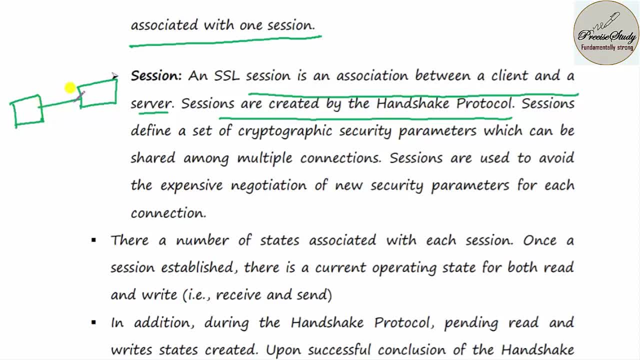 you'll be getting a notification that his call has been established, So you both can interact easily. So this is what I mean by handshake protocol. So there are a number of states associated with each session. Once a session is established, there is currently operating. 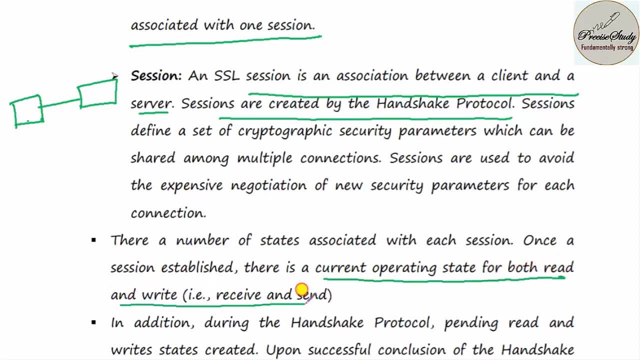 state both for read as well as write. Say, suppose the connection has been established, you can receive the data or you can transmit the data. Similarly, this person also can transmit the data or receive the data. So your telephone call falls under full duplex communication. 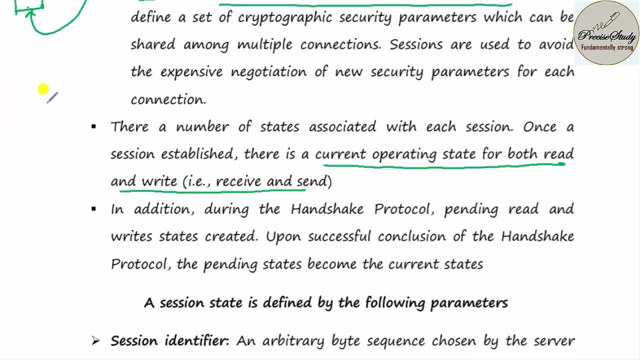 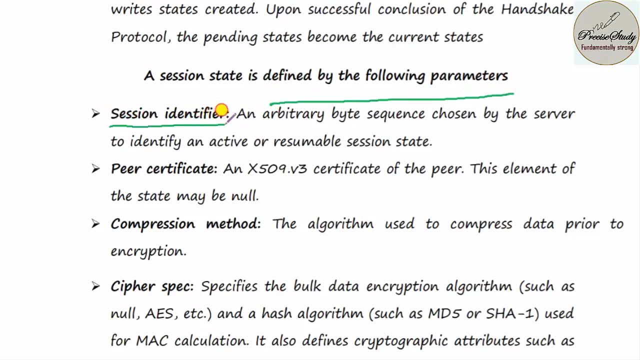 What do you mean by full duplex communication? It means simultaneously two persons can interact. The session state is defined by following parameters: The first one is session identifier. Second one is a peer certificate. Third one is compression method. Fourth one is cipher spec. 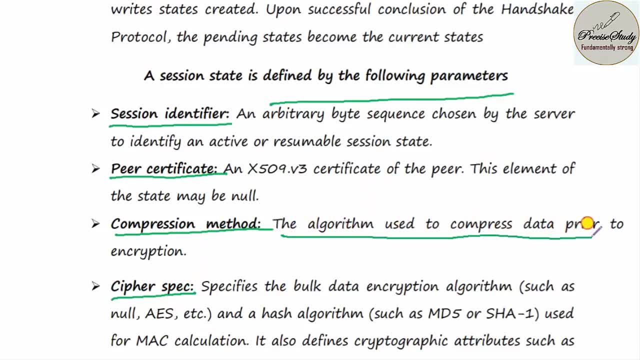 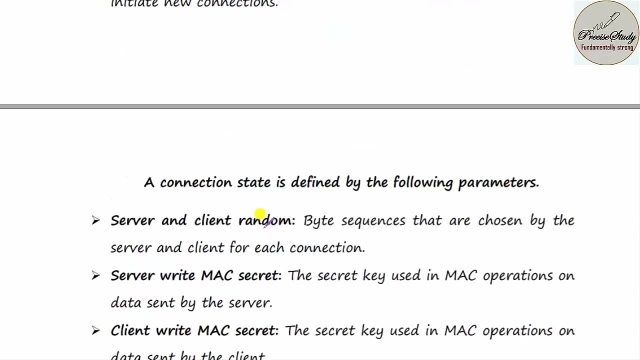 So what do you mean by compression method? Means the algorithm used to compress data prior to encryption. So why we are going for encryption means. Encryption means for secure data transmission. Compression is used to reduce the bandwidth of the particular user. So, apart from this, you will be having server and client random server. write. 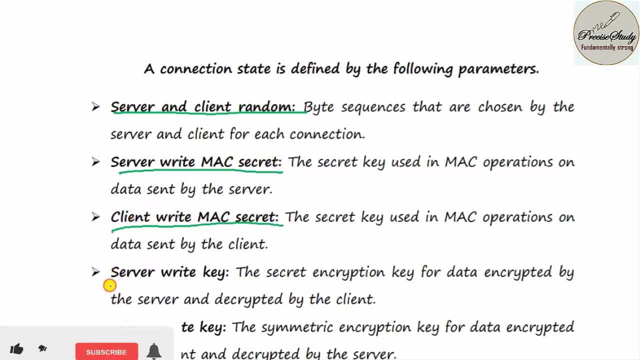 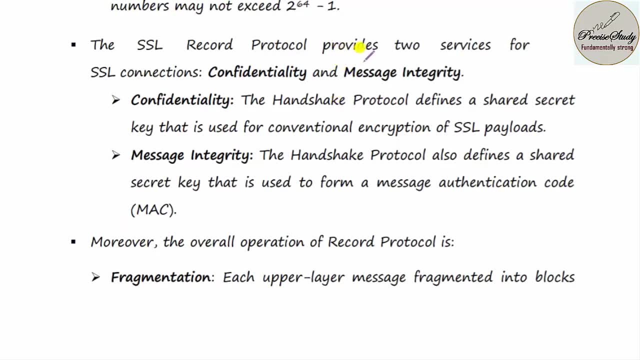 MAC secret client: write MAC secret server. write key client: write key. All these things, you can just go through it. The SSL record protocol provide two services for SSL connections. The first one is confidentiality and the second one is message integrity. They can ask you write a short note. 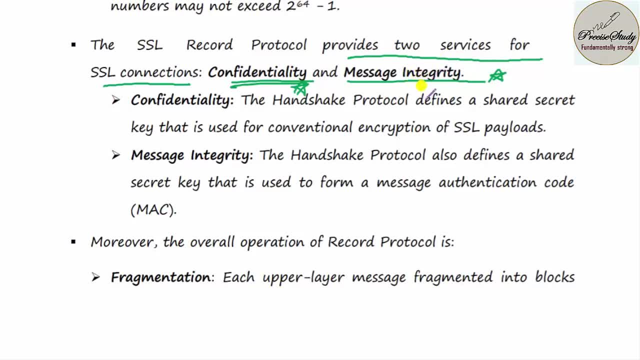 on confidentiality and message integrity. What do you mean by confidentiality? Means the ad check protocol defines a shared secret key that is used for conventional encryption of SSL payloads. Say suppose you both are communicating via phone call, So a network operator will be giving a confidentiality. 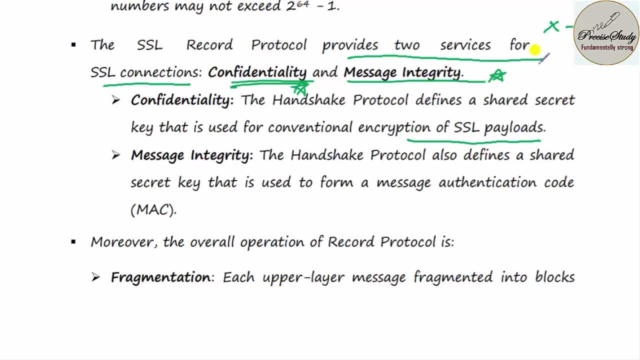 What he states is: your voice data will not be hacked by a third person. This is the amount of confidence that will be given by your network operator. So what do you mean by message? integrity Means the ad check protocol also defined a shared secret key that is used to form. 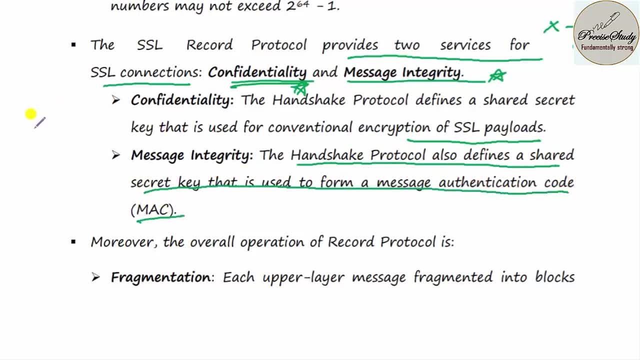 a message authentication code that is MAC. Say, suppose you want to do an internet transaction at that time The operator. what you will do is you will send an OTP. nothing but two step verification. the same key if you are putting back in the website. 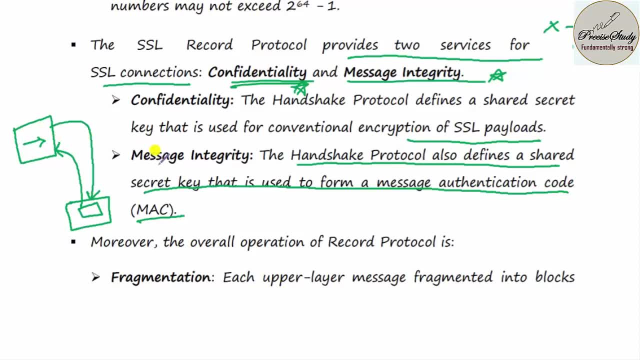 then next step will be processed. This is what you mean by message integrity. Moreover, the overall operations of the record protocol is fragmentation. What do you mean by fragmentation is So you'll be having a large memory. You're going to break into small, small pieces. 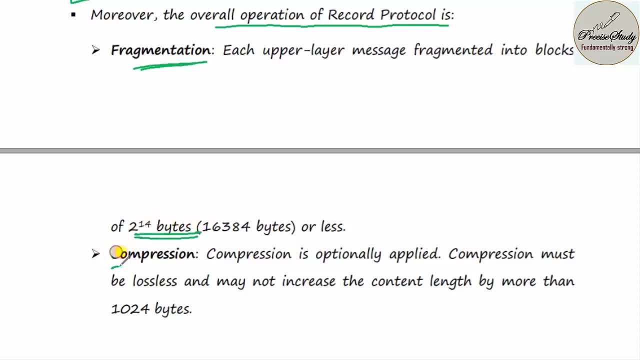 How many pieces you're going to do is 2 power 14 bytes. What do you mean by compression? So, for this example, is Winzip. So what are you going to do? is you're going to reduce the data bit size? 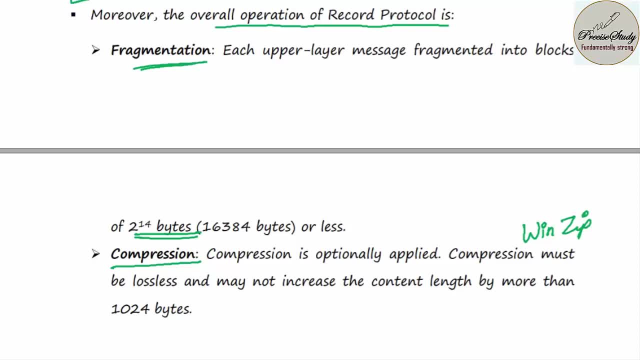 So what are you going to do is actually? you're going to compress your data. Compression will be done such that there will be no any losses. So this compression, I can relate with respect to decimation. I can relate with respect to decimation. 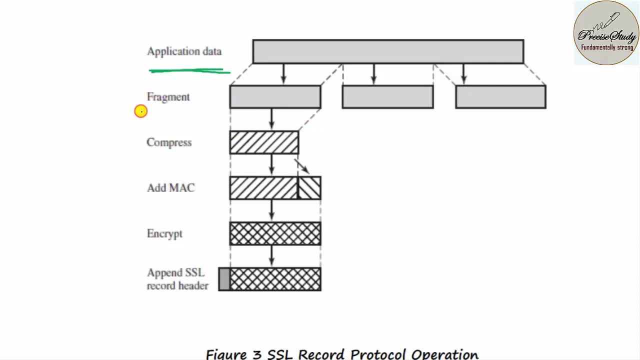 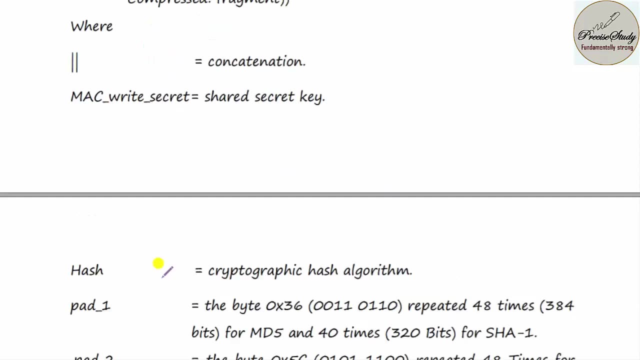 So, first one, you'll be having application data. Second one is fragmentation. Third step, you'll be doing compression. Fourth one is add MAC. Fifth one is you're going to perform encryption. And the seventh step is: append SSL record header And then you're going to transmit the data. 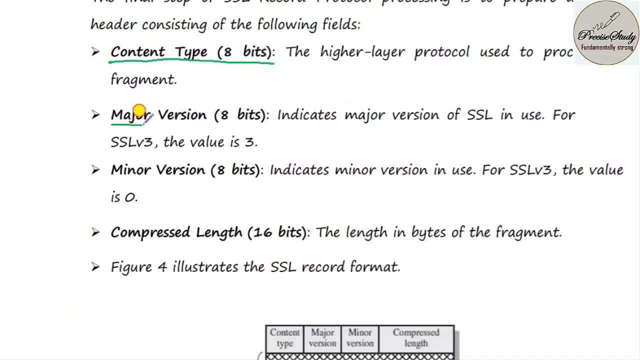 So the content type can be of 8 bit, Major version is of 8 bit. Minor version is also of 8 bit. Compressed length may be of 16 bit. Let us talk about server authentication and key exchange. What do you mean by server authentication and key exchange means? 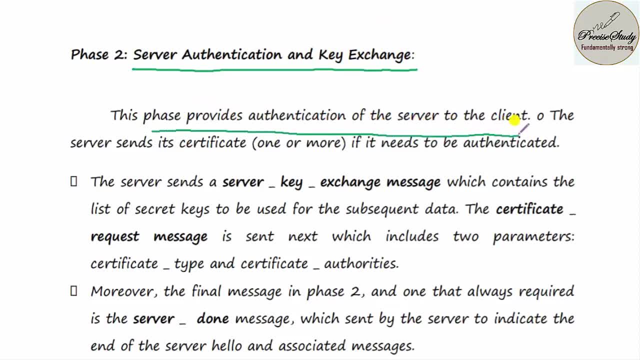 It provides authentication of the server to the client. The server sends it certificates, that is one or more if it needs to be authenticated. So suppose if you are opening some website so they will be telling it SSL certificate, So you can view their SSL certificate. 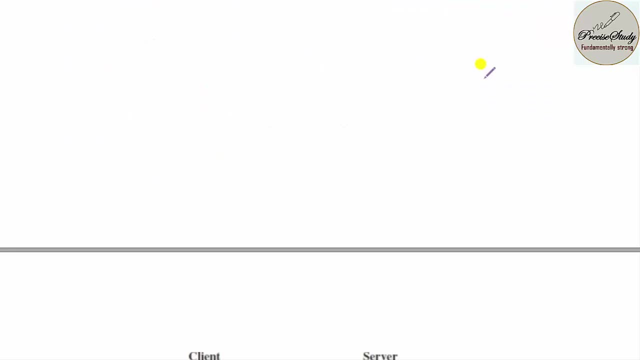 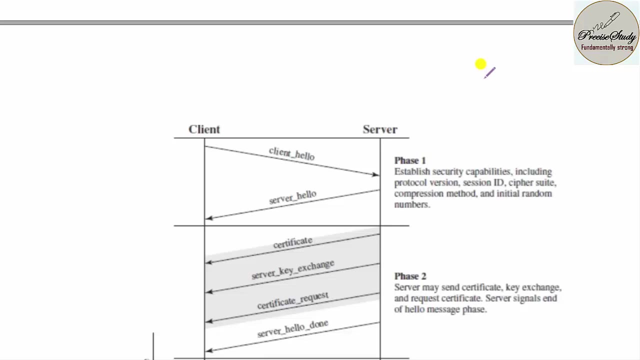 Nothing, but it is a secured website. So some of the fake websites also will be there. So those websites, what they will do is they will not be giving any security measures. that will be start from HTTP. If it is a secured website, then it is HTTP. 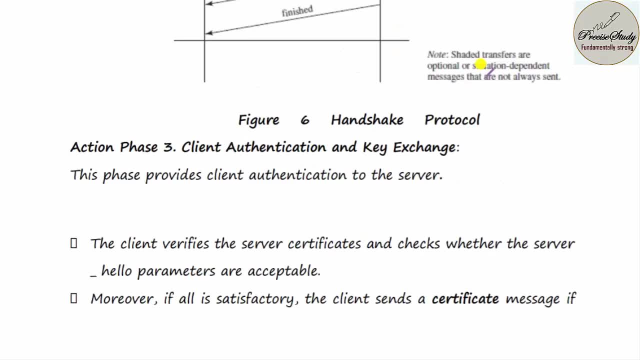 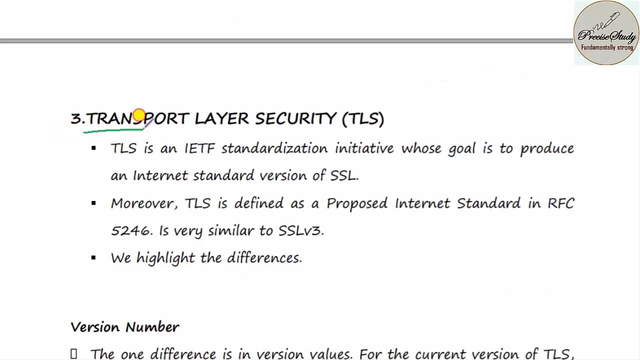 Yes, nothing but one extra level of security They will be giving in the case of HTTPS website. So next topic is transport layer security. So it is a IETF standard and it is an initiative whose goal is to produce an internet standard version of SSL. Moreover, transport layer security is: 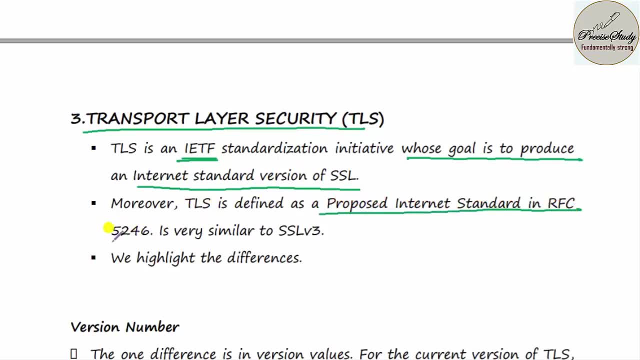 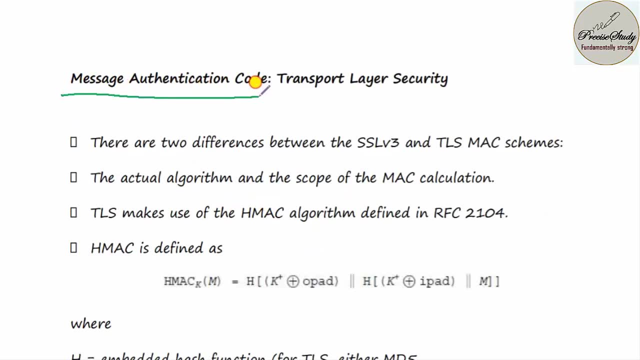 defined as a proposed internet standard in RFC 5246. It is similar to SSL version 3.. So what do you mean by message authentication code? in the case of transport layer security, There are two difference between SSL version 3 and TLS MAC schemes. 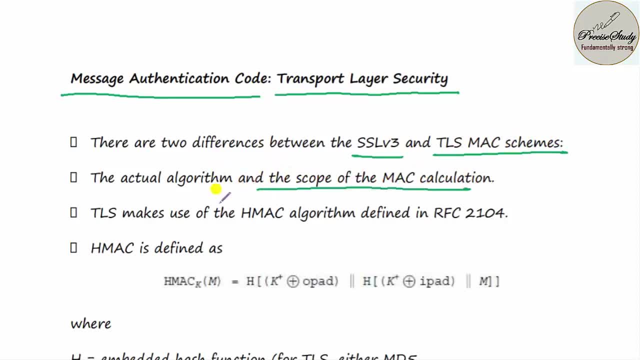 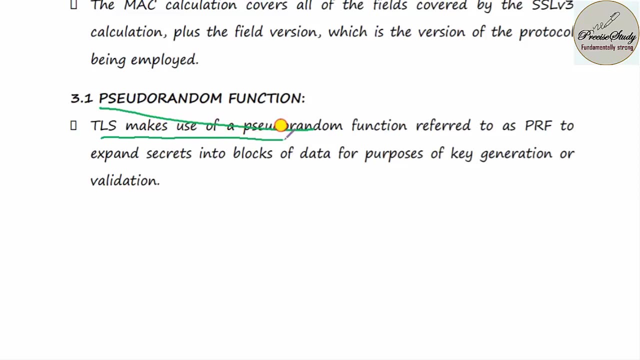 So the actual algorithm and the scope of MAC calculation. and the second one is TLS makes use of HMAC algorithm defined in RFC 2104.. Next, let us talk about pseudo random function. What do you mean by pseudo random function? is TLS makes use of pseudo random? 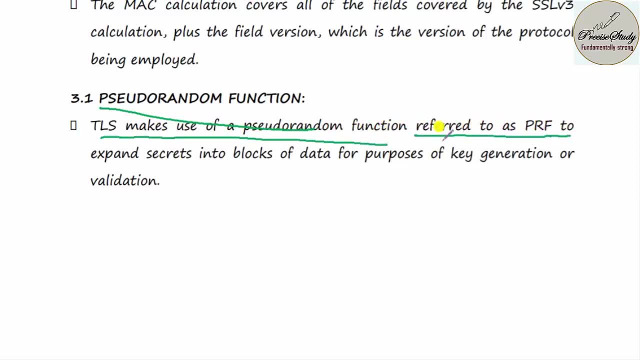 function, referred to as PRF, to expand secrets into blocks of data for purposes of key generation or validation. So this pseudo, random sequence you have studied in your digital communication, You, what you are going to do is you are going to make use of frequency hopping. 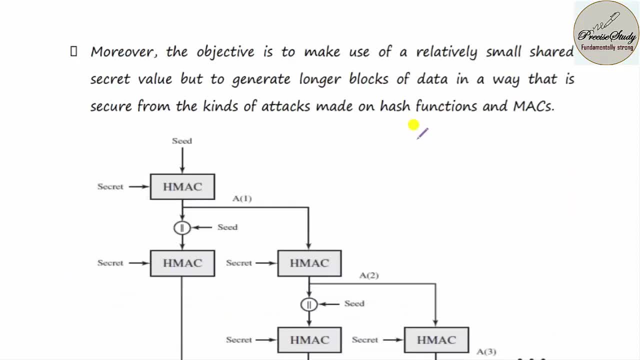 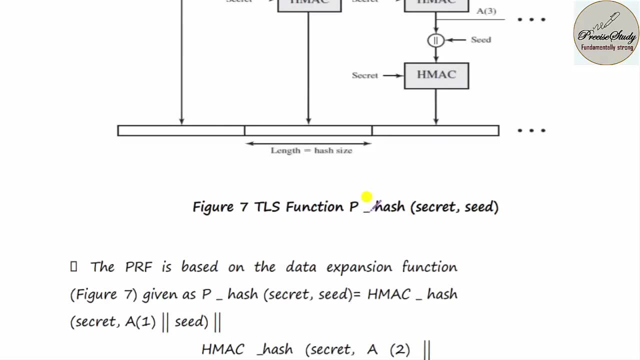 techniques, nothing. but instead of using one carrier, you are going to make use of multiple carriers and some random numbers you are going to generate as a carrier. That is what you mean by pseudo random sequence. Next, let us talk about transport layer security. 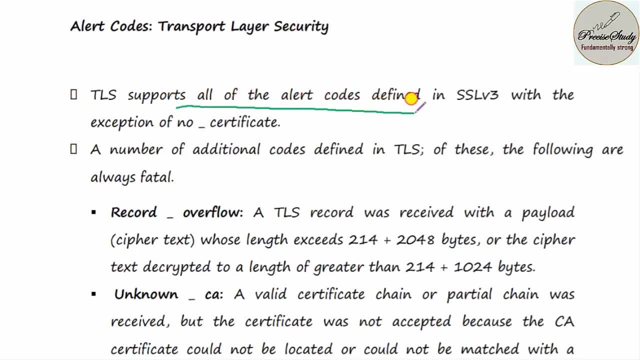 Transport layer security supports all of the alert codes defined in SSL Version three, with the exception of no certificate. the number of additional codes is defined in TLS. of this, The following are always fatal. fatal means always there will be an error. So the first one is record overflow and the second one is unknown. 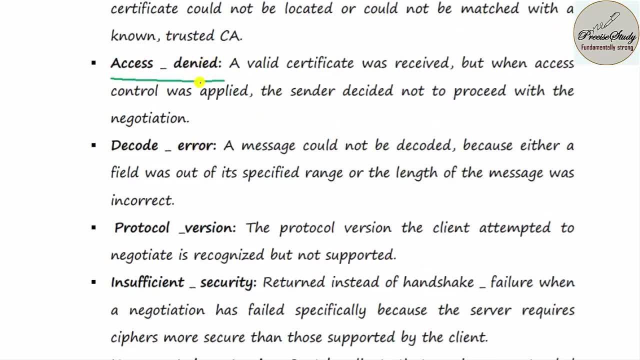 The third one is access denied. Say suppose, if you want to access any of the military website and if you want to modify, then you'll be getting an error as access denied decode error. simple example of access denied is: say suppose your friend is having a cell phone. 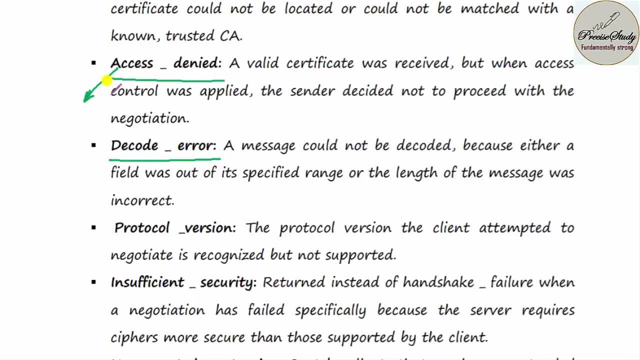 So, without his knowledge, what do you do? is you try to open the pattern lock? If you're not knowing the pattern lock, it will be throwing an error as a wrong pin- Wrong pin- indicates it is access denied. Next you need to talk about protocol version, insufficient security. 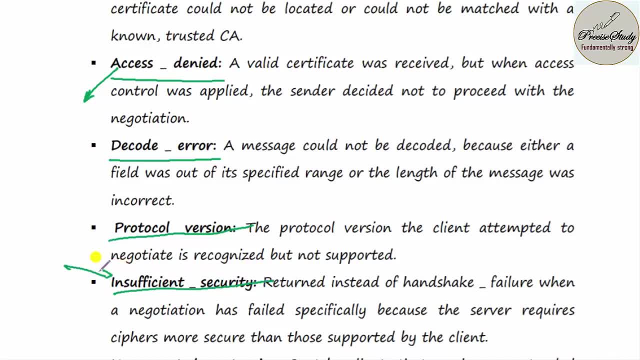 Insufficient security means, say, suppose, you have created a new Gmail account. You try to keep the password as A123456.. So what? it is going to throw an error as insufficient security. or you can keep it as ASZ1234. Or you keep the password as ASZFZXCV. 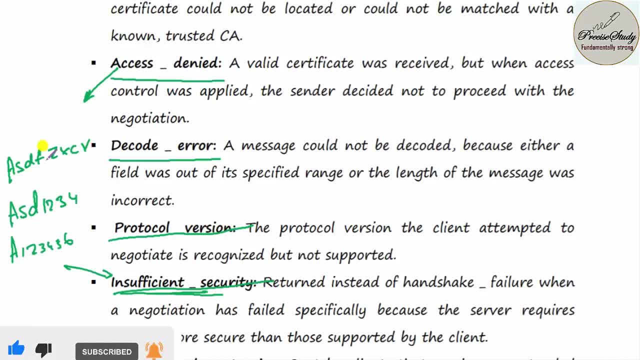 What actually many of the websites will recommend is the password should contain one capital letter, one small letter, one number, one alpha character. So total number of characters should be minimum eight. they will be asking. So that's how they are going to give the. I. 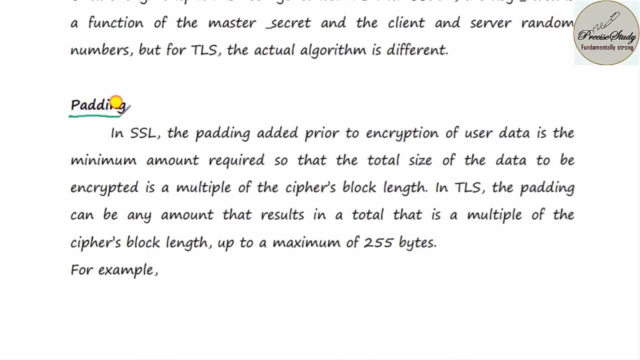 security for the user. Next, let us talk about padding. So, in order to explain the padding concept, so I'll be going with n comma, k coding. So where k is the number of data bits, n is the total encrypted bits or total. 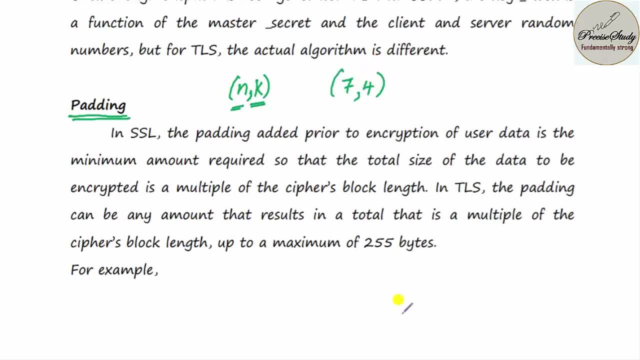 number of bits with encryption. say suppose I'm going with seven comma four code, So you'll be having four data bits and you'll be having three parity bits. So this four data bits, I'm going to represent it as D3, D2, D1, D0.. 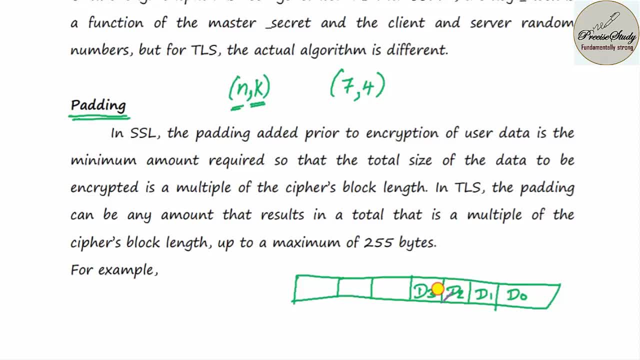 So in order to judge the change in the data bit, So what are you going to do? is you're going to make use of the parity bit, that is, P2, P1, P0.. So what is the value of P0, P1, P2 is given by the XOR of the particular data bits. 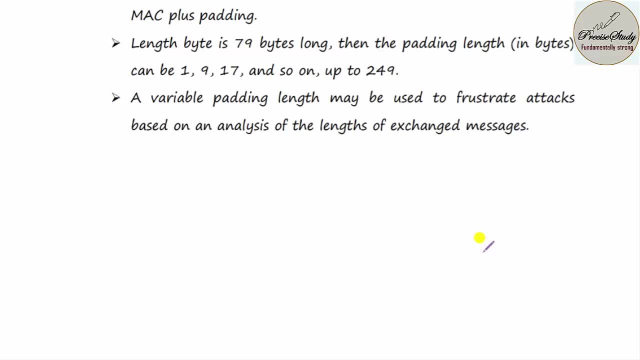 So this is what I mean by padding, Especially if you want to increase the clarity. what you're going to do is you're going with interpolation. There are four variants of interpolation. The first one is zero interpolation. The second one is unit step interpolation. 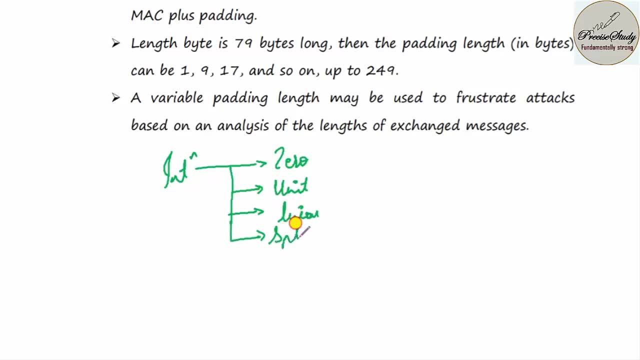 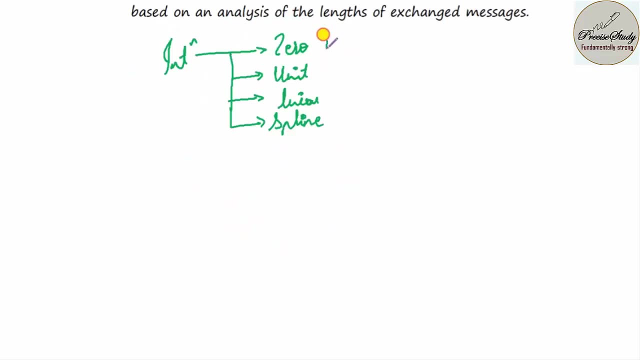 And the third one is linear interpolation And the fourth one is spline interpolation. So in the case of interpolation, you may add zeros, or you may add the previous digits, or you may add the average of the next sample and the previous sample. So this is what we mean by interpolation: nothing but you're going to add. 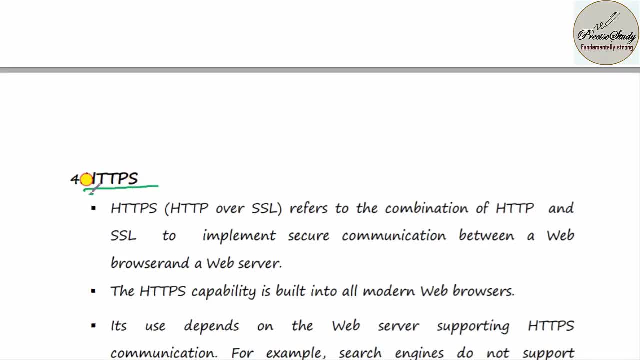 zeros. What do you mean by hypertext transfer protocol with SSL security, Say suppose I'm considering some website, say HTTP. The particular website is there dot com, So this website is not secured. I'll be considering one more website: HTTPS colon www dot precise study dot com. 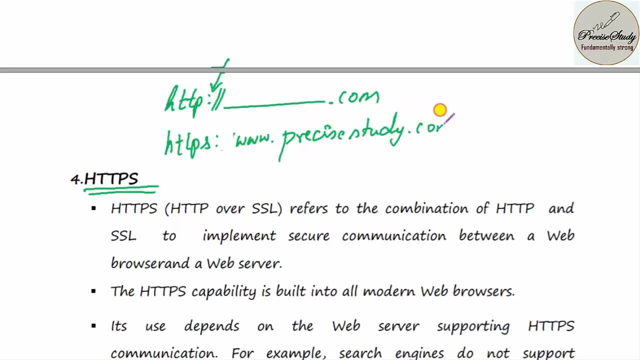 So in this website this person has paid some amount for extra security, I think. but whatever the contents he'll be posting on his website, some other person should not post because he will not be knowing the password and he should not be in a position to add the data. 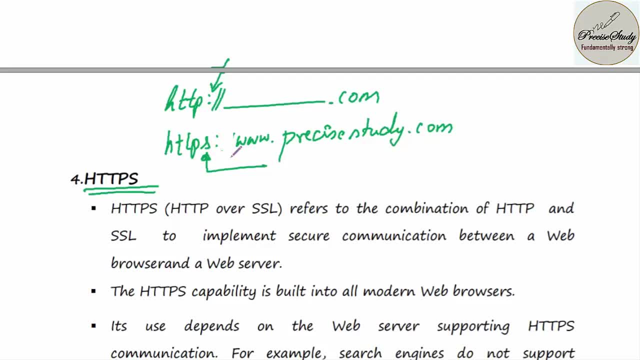 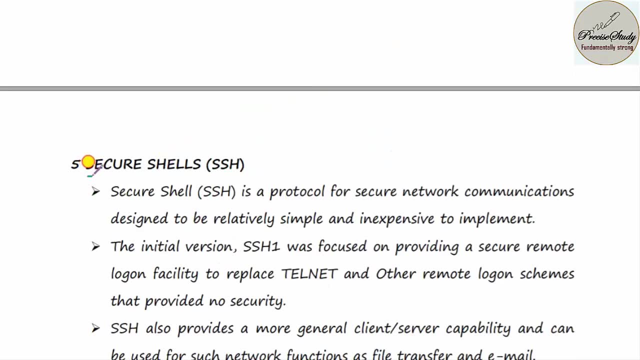 Nothing but one extra level of security you're going to provide by expecting some money from the user. The main thing is they'll be asking you write a short note on secure shells, That is, SSL. secure shell is a protocol for secure network communication, designed to be relatively simple and it is inexpensive to implement it. 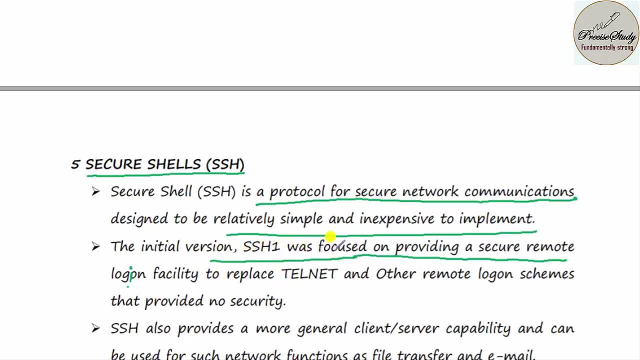 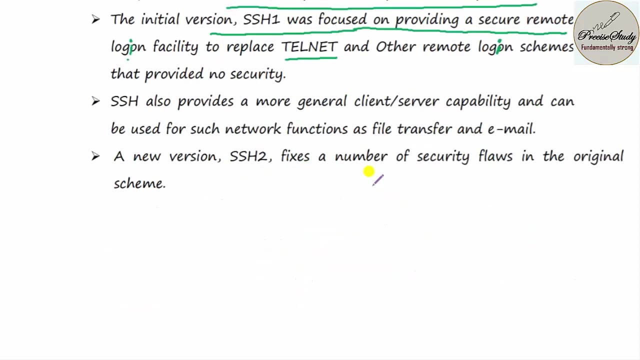 The initial version, that is, SSL one, was focused on providing a secure remote login facility to replace telnet and other remote login schemes. that provides no security. SSL also provides a more general client server compatibility or capability and can be used for such network functions as file transfer and email. 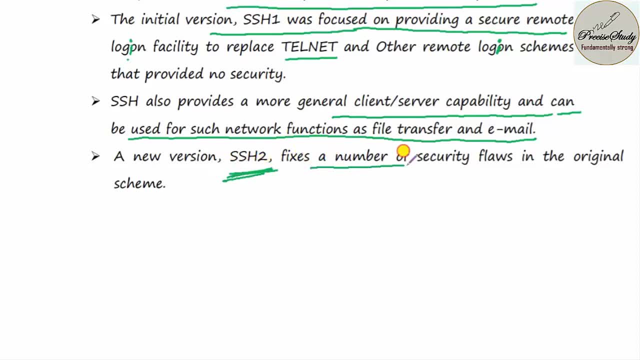 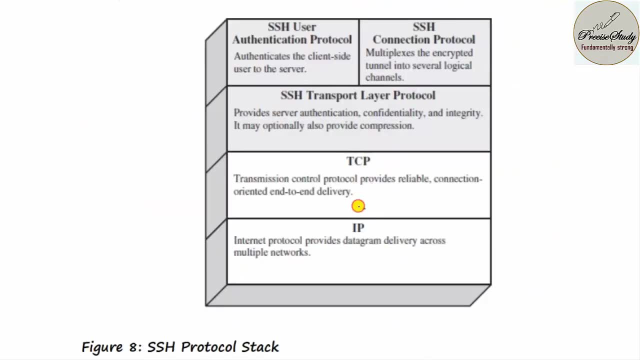 The new version is SSH2.. It fixes a number of security flaws in the original scheme. The protocol stack, as I discussed, in the first layer will be having internet protocol and the second layer will be having TCP protocol and third layer will be having SSH transport layer protocol and the fourth one is SSH user. 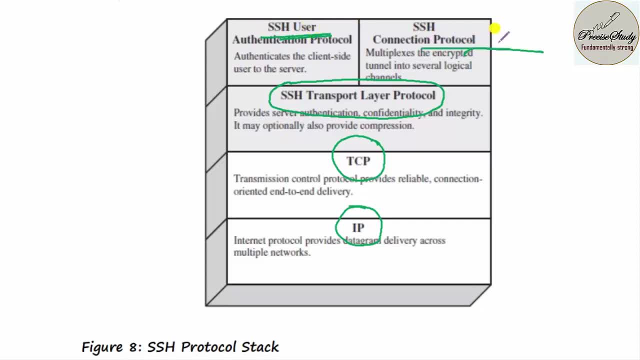 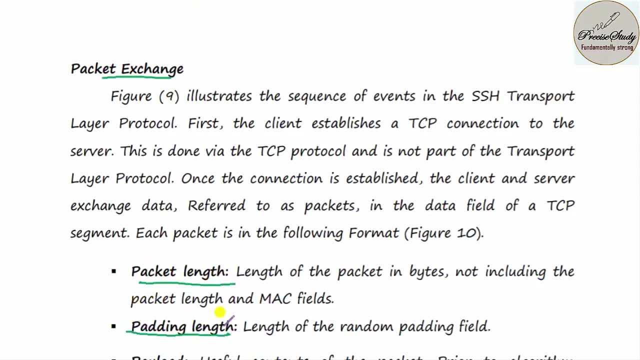 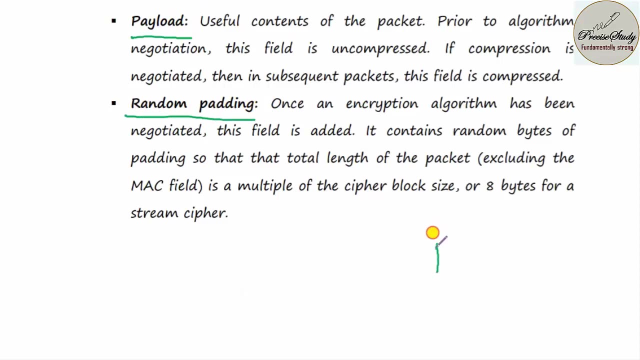 authentication protocol or connection protocol. So these things are important. Next, in the package exchange, we need to talk about what is the package length, what is the padding length. also, we need to talk about payload and random padding. So if I'm considering four bits of data, 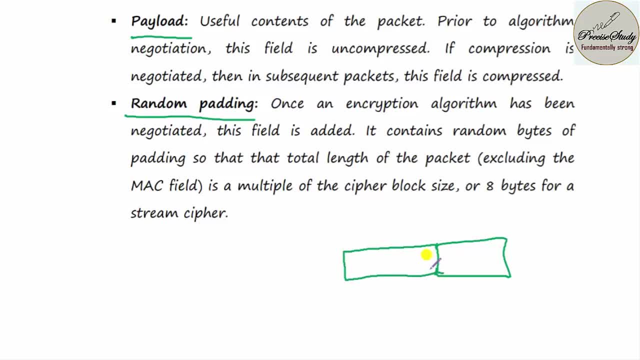 so for this you can't pad more than two or three bits, because your data bit should be more and your encrypted bits should be less in number. But in the case of military, what you're going to do is your data is of less bit. error correcting. 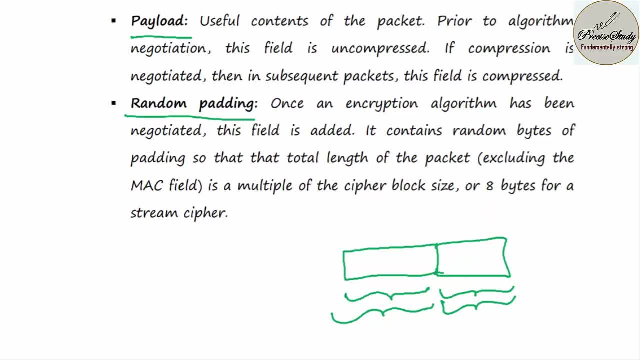 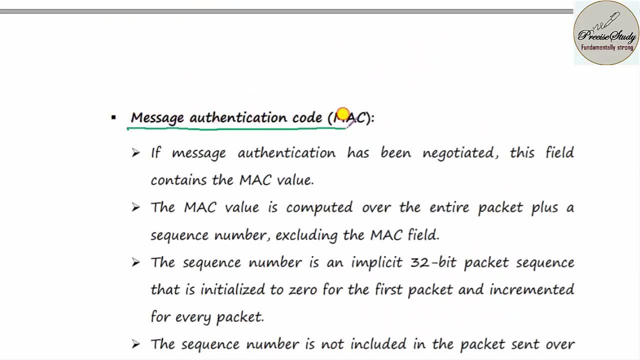 Bits will be more in number when compared to data bits. It all depends what type of communication you are doing. Next topic is message authentication code. If message authentication has been negotiated, this field contains a MAC value. The MAC value is computed over an entire. 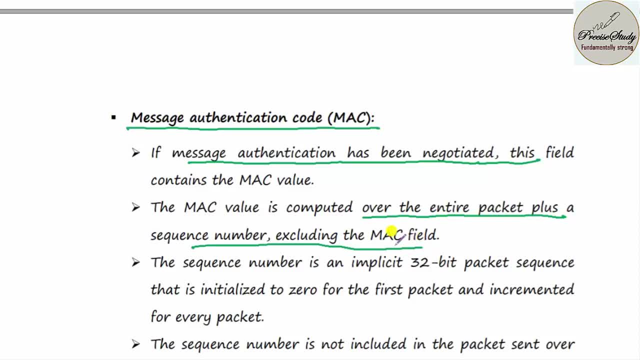 packet plus a sequence number, excluding the MAC field. The sequence number is an implicit which is of 32 bit packet sequence that is initialized to zero for the first packet and it is incremented for every packet. Say suppose, in the case of digital electronics, if I'm telling mod 15 counter. 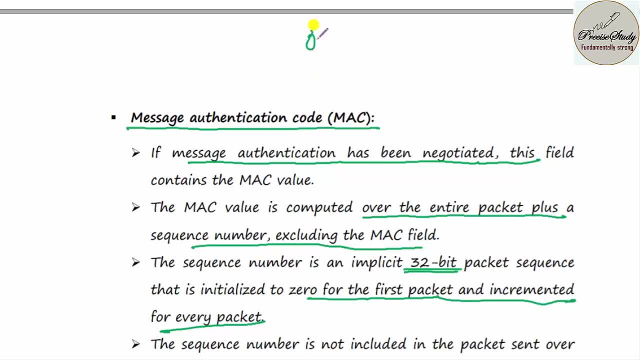 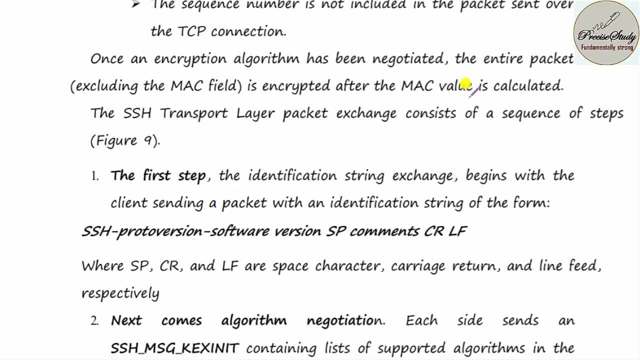 so your counter will be counting the sequence from 0,, 1,, 2,, 3,, so on to 14.. So it is going to include zero. The SSH transport layer packet Exchange consists of sequence of steps. The first step is identification of string. exchange begins with the client sending.